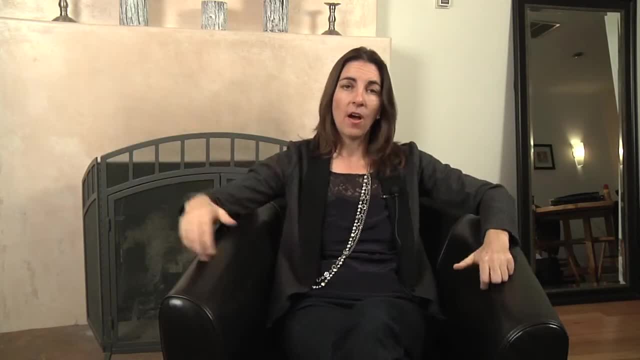 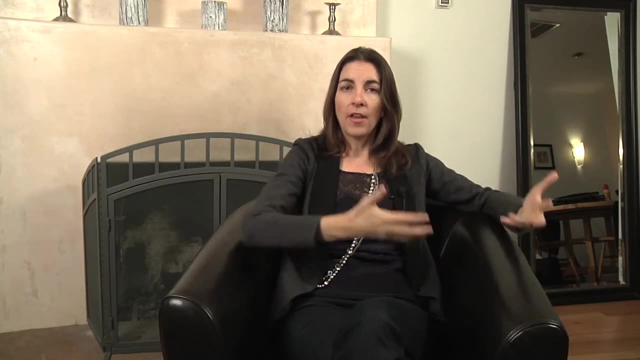 real hard classes And, in fact, the grades tend to drop off. by the time they get into high school, The scores go down. Well, why is that? Well, we haven't really prepared our young kids, our elementary students and our middle school students, to be able to take 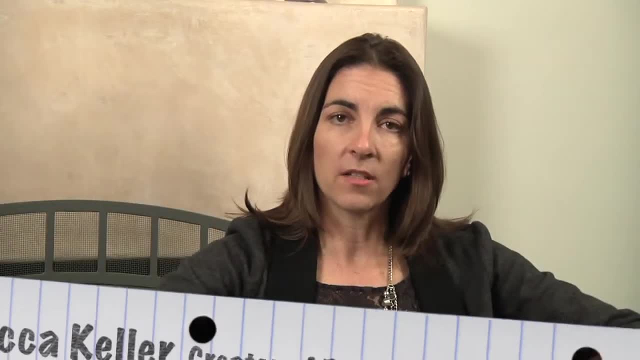 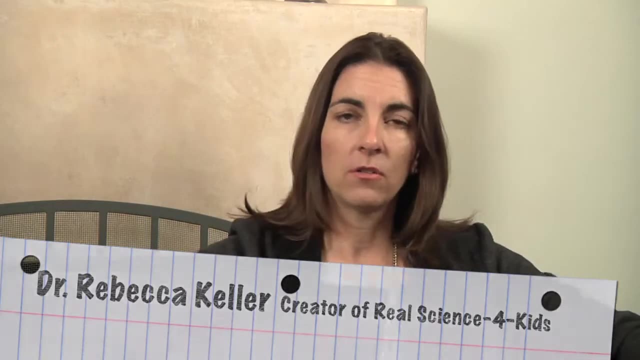 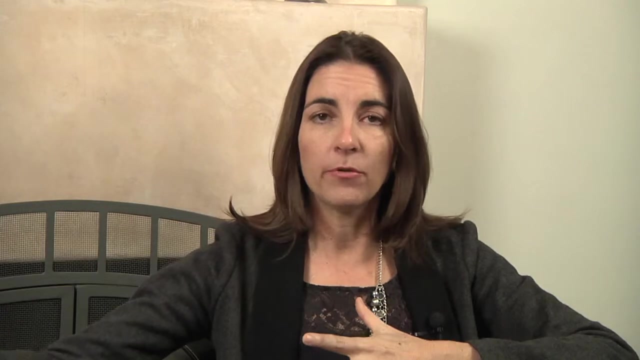 on chemistry and physics in high school, So I wrote Real Science for Kids Starting with kindergarten or first grade. my pre-level chemistry introduces very young students to the concepts of atoms and molecules and chemical reactions and acids and bases and polymers and DNA and protein. These are the subjects that a student will be exposed to, will have 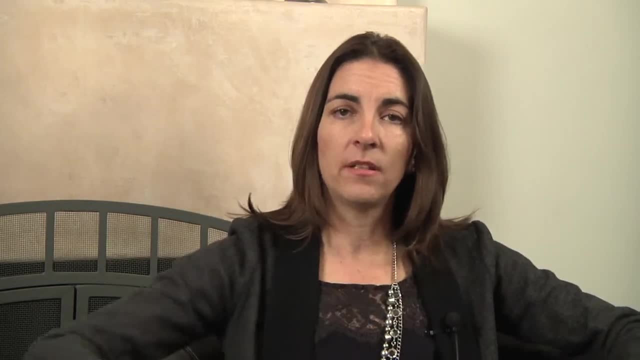 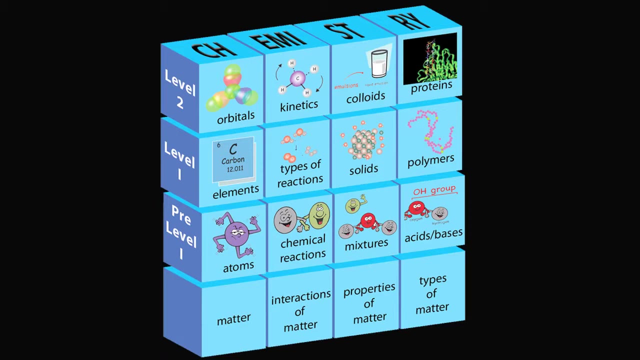 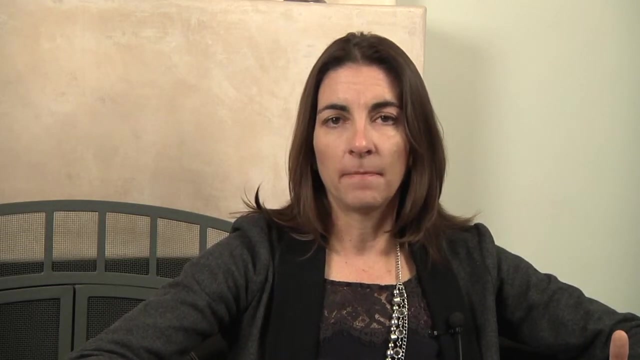 to learn in high school And then in my level one series I teach kids the same subjects, the same topics- atoms and molecules, and chemical reactions and acids and bases, and proteins and polymers- And the idea here is that learning science, in my opinion, is no different than learning a language. 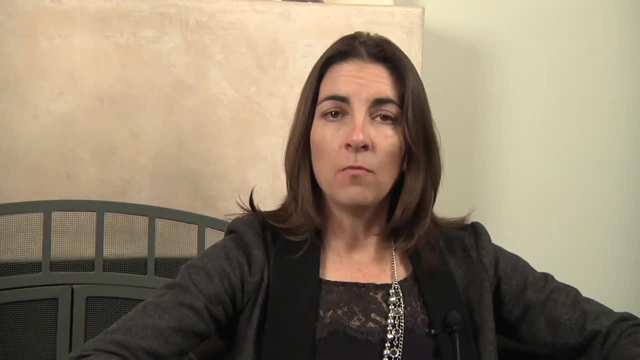 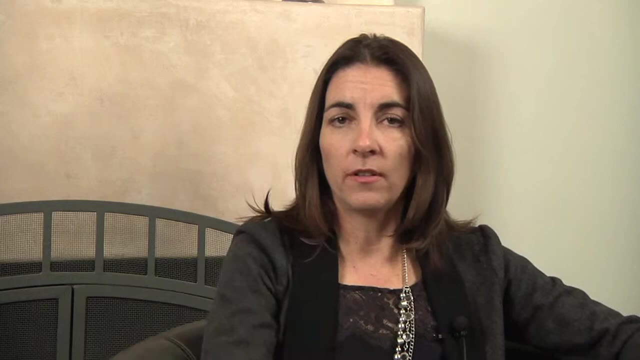 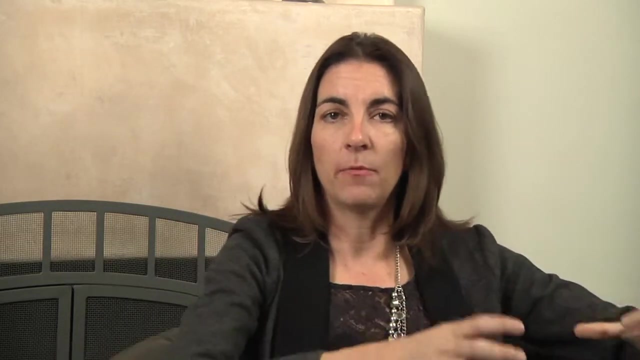 or learning math or learning music. You must expose kids to the foundational building blocks for the subject that you want them to know, And so, in When we learn a language, we introduce kids to the alphabet and then to you know how to make words from the letters of the alphabet and how to put words together to make sentences. 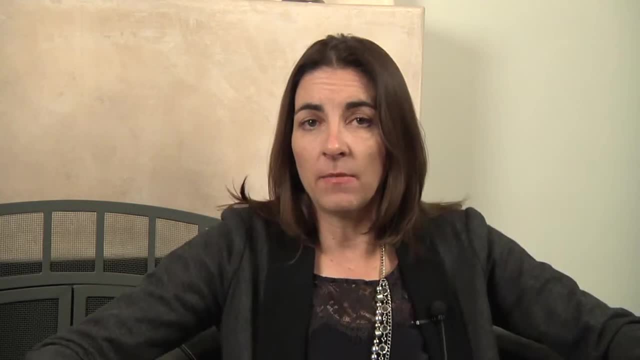 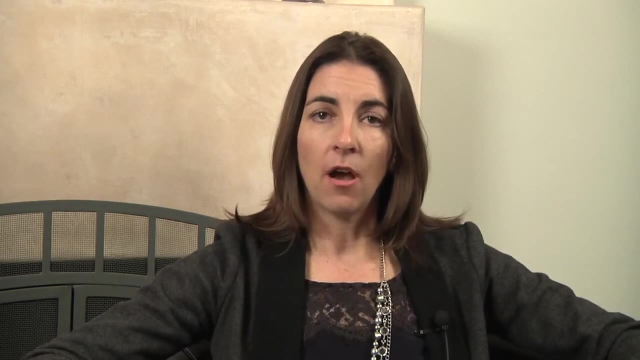 and so on. We give them the building blocks of language. The same is true with math and music, And so why not do this for science? Why not give students the building blocks for real science? Give them the chemistry, give them the physics, give them the biology. 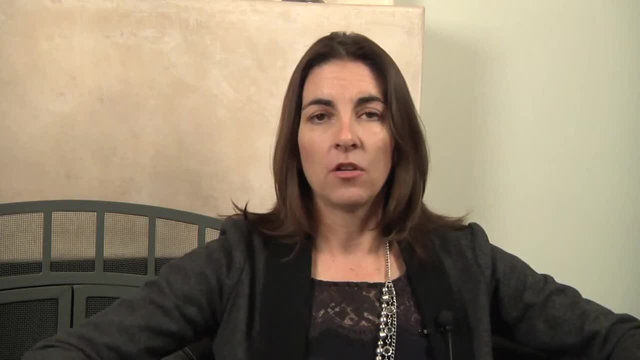 the real biology, which is really applied chemistry and physics to a living science. And so we give kids the real science, the real science that they're good at, but you give them the real science that is actually favorable to a living system. So now that they know, 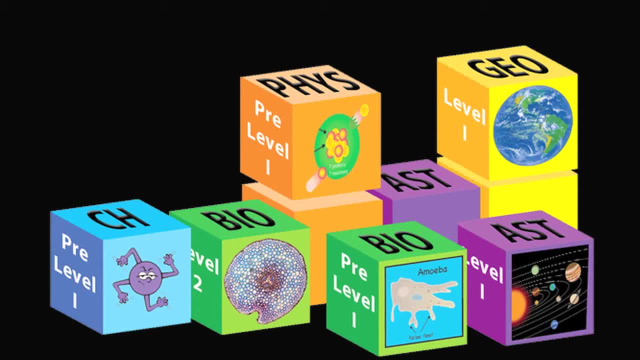 the chemistry and physics. you can start talking about the chemistry and physics of living systems and biology, and then you can go on to discuss the chemistry and physics of nonliving systems in geology and astronomy, And in my mind, this is the way to lay a solid foundation.